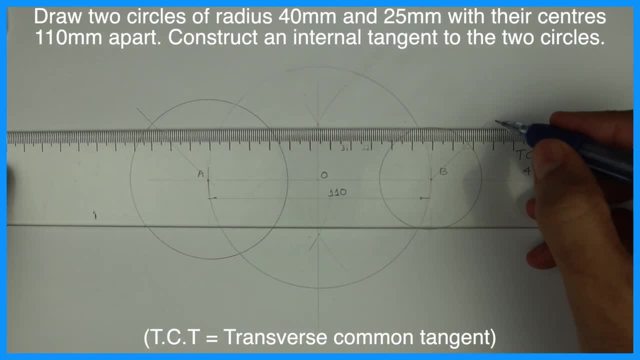 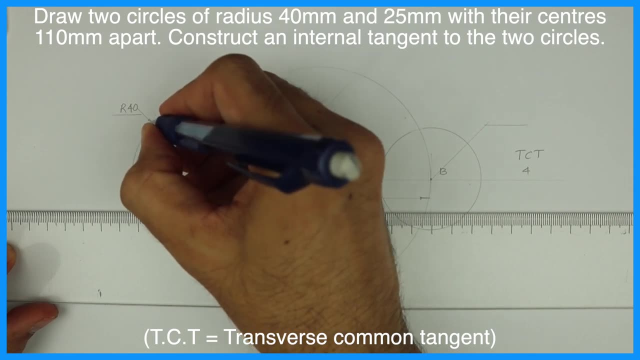 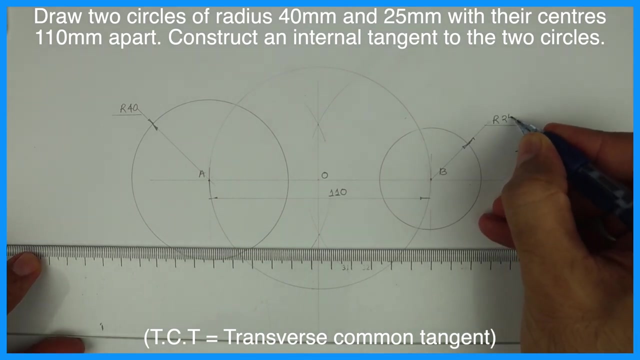 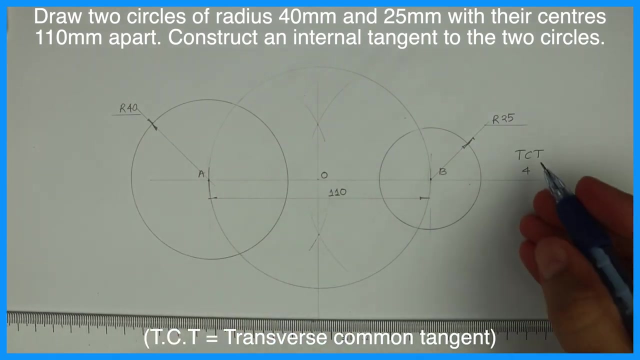 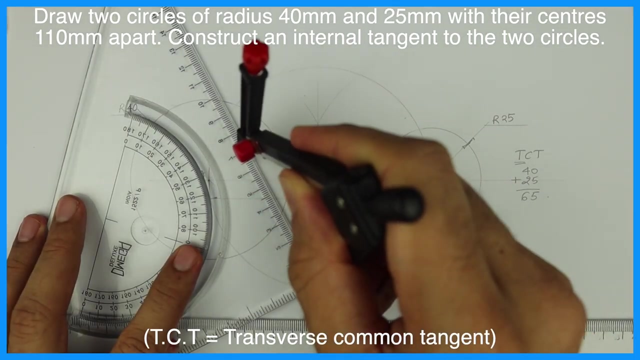 40 and this is radius 25.. So total would be 40 plus TCT. So this is TCT, this is radius 25.. So that is 65, so you take 65 in your compass and you draw it from A. you can draw it from. 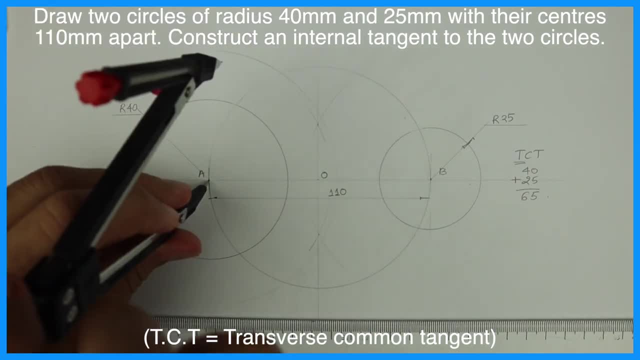 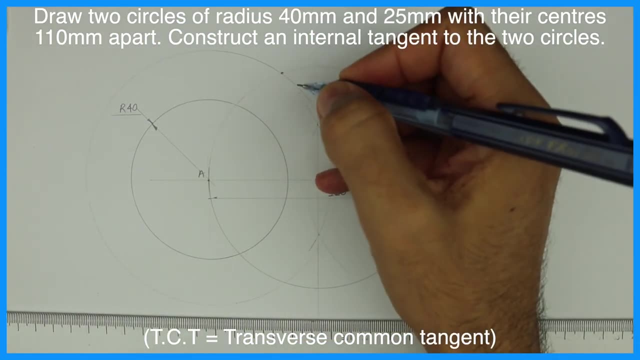 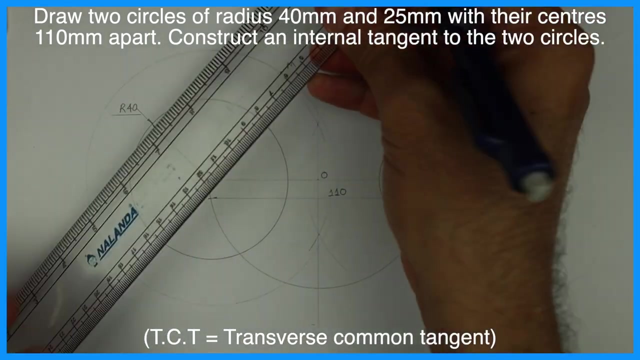 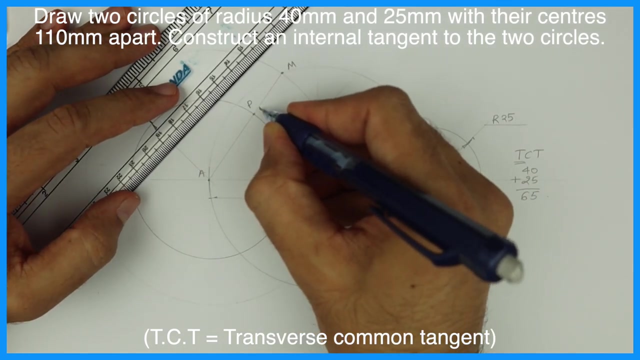 B also, but we will keep it constant wherever it will cut with the middle circle. that mid circle, that is point M. now join A to M. wherever it will cut on the main circle, that is point P, and I will write T1.. 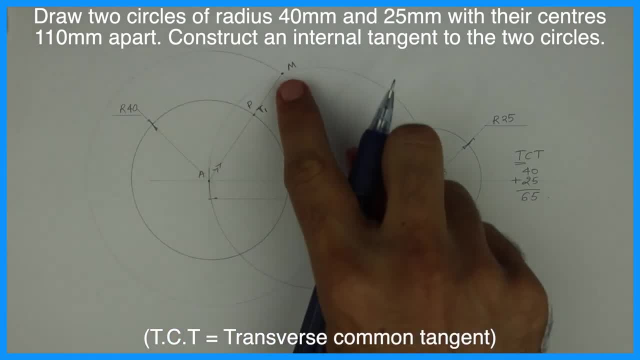 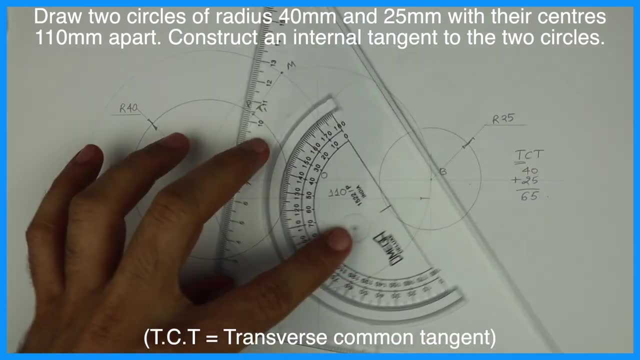 Now I need to draw parallel line to this. see this: A to M, point T1,. now we need to draw parallel to this, So we will draw this line from here. So we will draw this line from here. So we will draw this line from here. 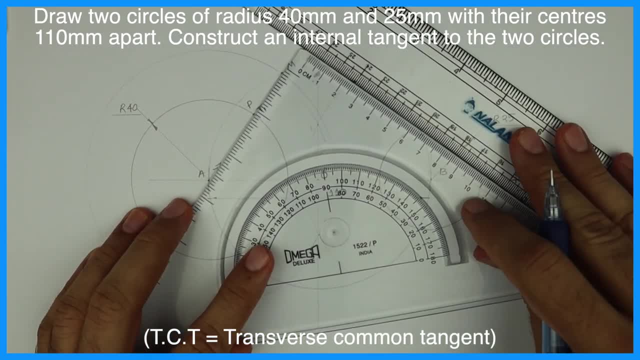 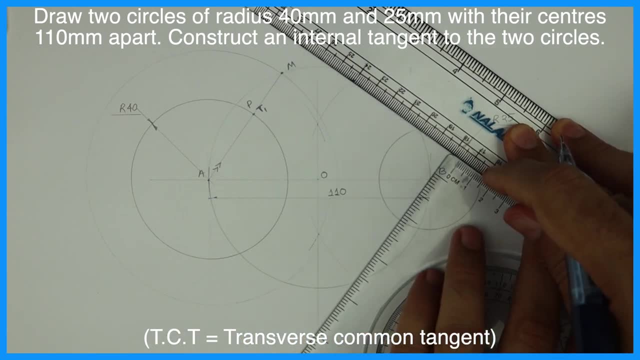 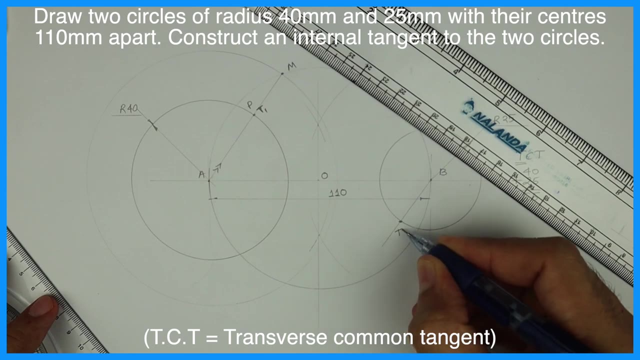 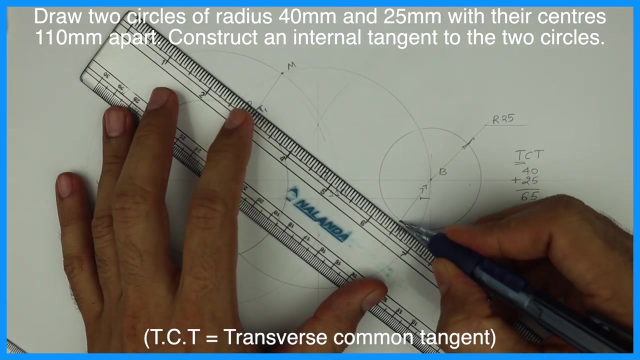 So we will get parallel passing through point B. see this, and we will draw parallel line and it should pass through point B, So we will get point T2.. Now we join T1 to T2, so this is internal tangent or Transverse Common Tangent. 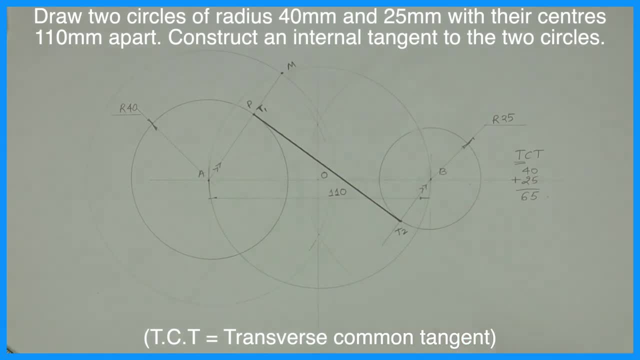 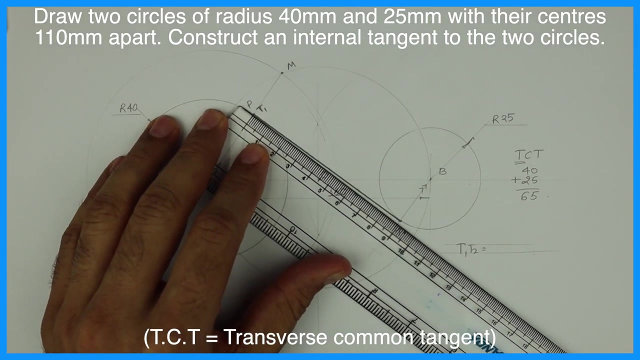 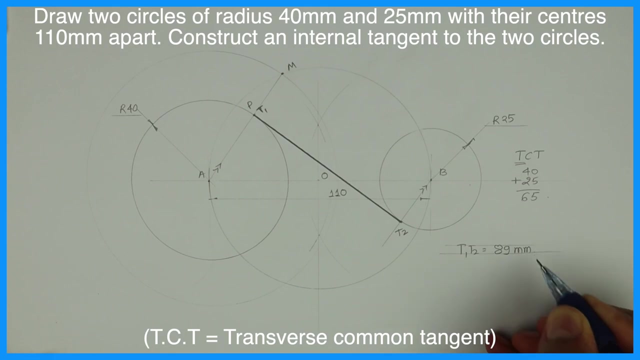 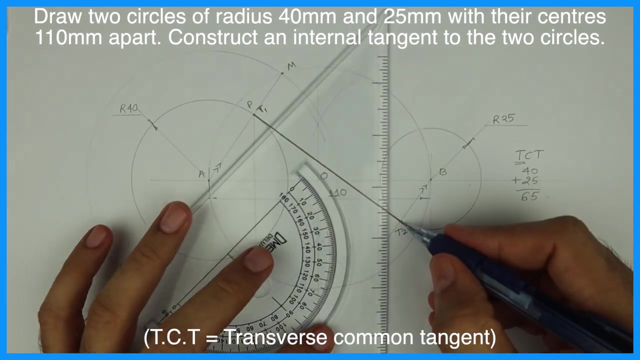 if they will tell you draw tangents or they want you to draw both the tangent, see, we can write t1- t2- value of t1- t2, 89 mm. and if they will ask you to draw both the tangents, then extend this point down and extend this point up wherever it will cut from that point to.